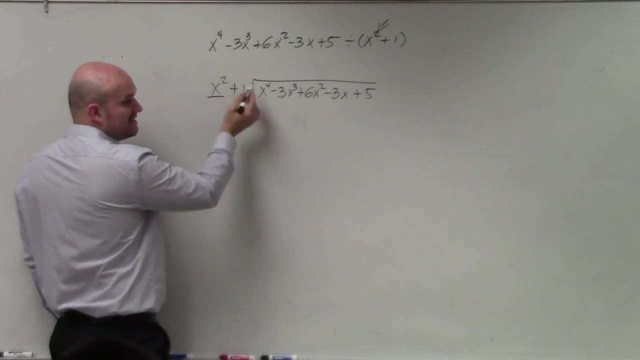 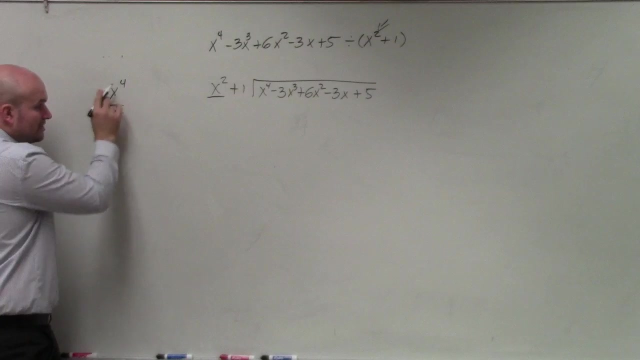 through my steps. you take x and divide it to x to the fourth. How many times does x squared divide into x to the fourth, If that kind of tricks you up again? I'm basically just asking: how many times does x squared divide into x to the fourth Using your rules? 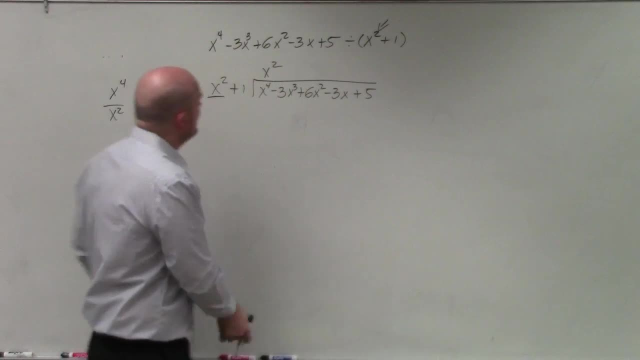 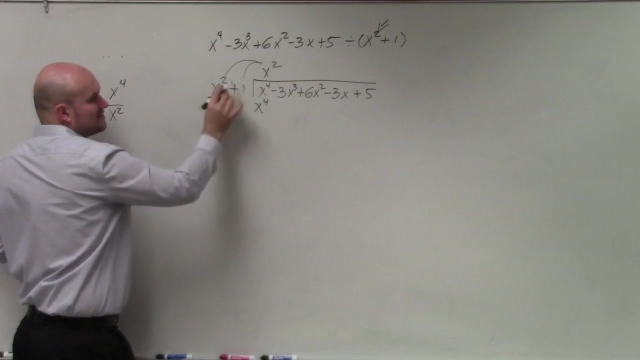 of exponents. you get x squared because you subtract the powers. Then I take this value, x, Then I multiply it by both terms. So x squared times x squared is x. to the fourth, x squared times 1 is x. Now I don't want to write that here because I can't subtract x, cubed and 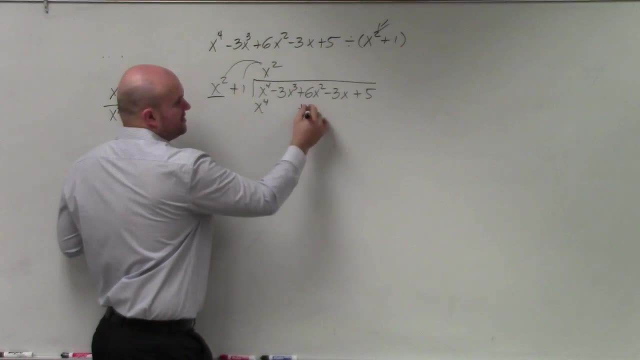 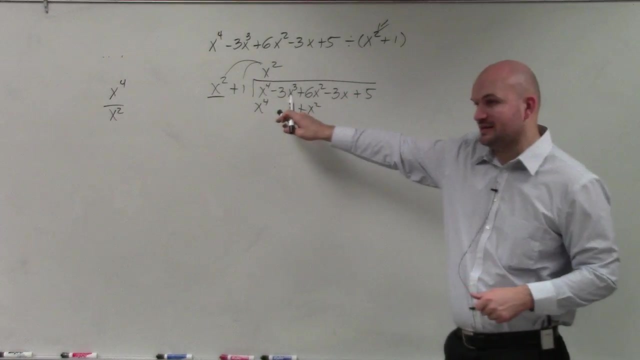 x squared. So what I need to do is I need to move that over here, because those are like terms. What I showed what you can do then if you don't like this space is you can put a space value there. You can put like a 0x cubed if you like. 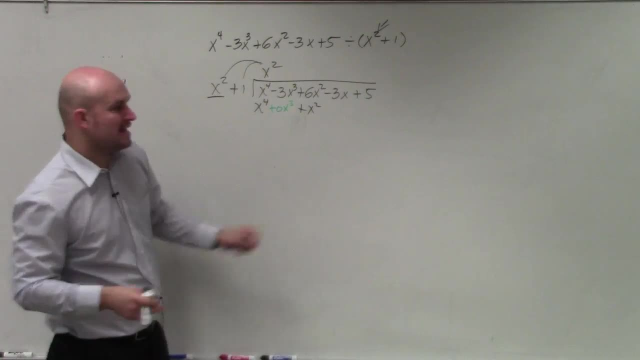 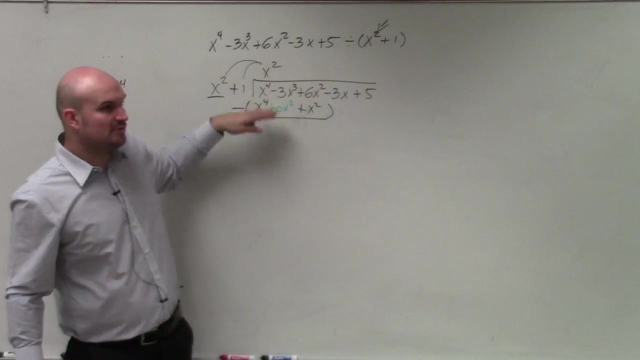 But what you'll notice is: it doesn't really matter, It's just going to go all the way down. Then the last step is you're going to subtract the rows. Make sure you put them in parentheses, because you've got to subtract both of these values, So you have x to the 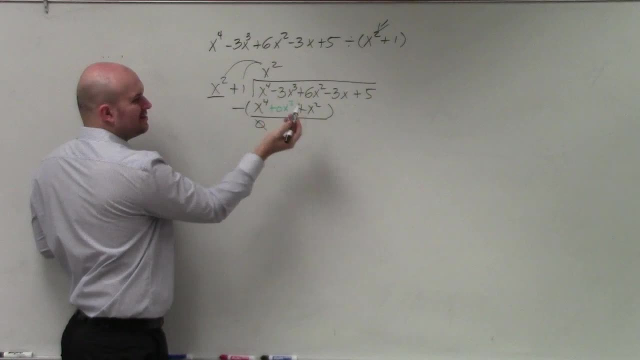 fourth minus x to the fourth is 0.. Negative, 3 minus 0, which you just realize is really just bringing it down, And then you have 6x squared minus x squared, which is a positive 5x squared. You could put zeros in for here, or you can just kind of realize that these 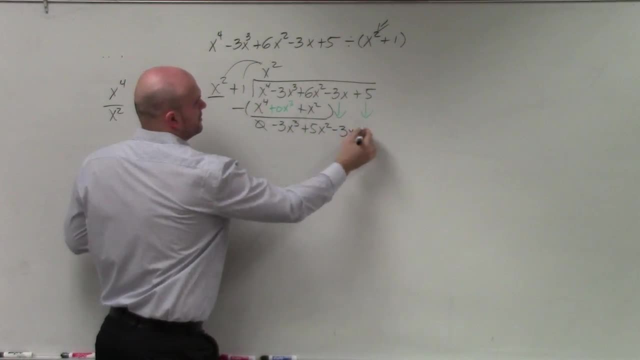 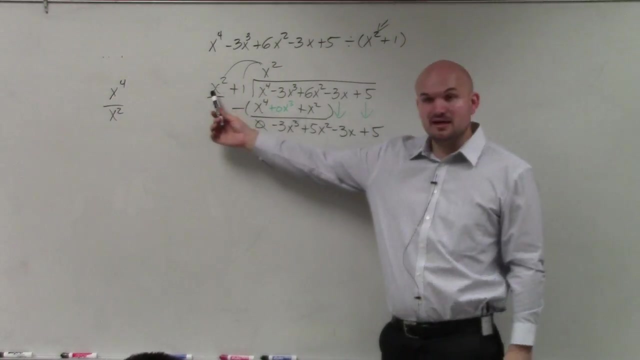 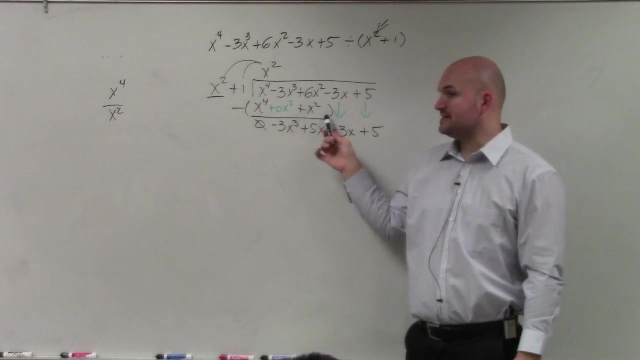 are both going to come down as well. Okay, So what I want you guys to understand is that is like one round. Basically what I did: I took the first term, divided it into the first value, put my quotient answer, multiplied it by both of them, wrote that down and then subtracted. So I divided, multiplied and 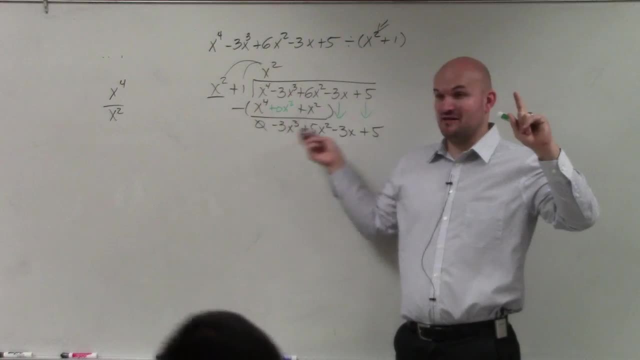 then subtracted, That's one round. Well, guess what? I still have more rounds to go. So now, basically, what you do is just do it all over again. How many times is x squared going to negative? 3x cubed? 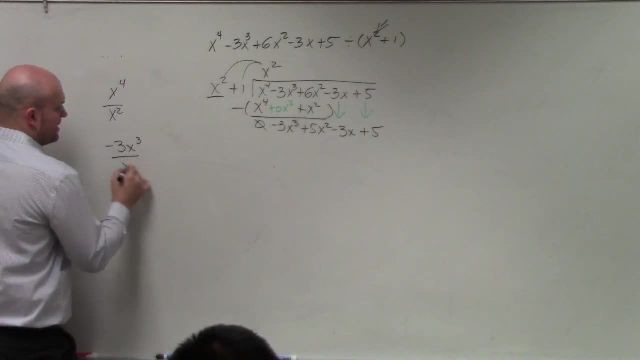 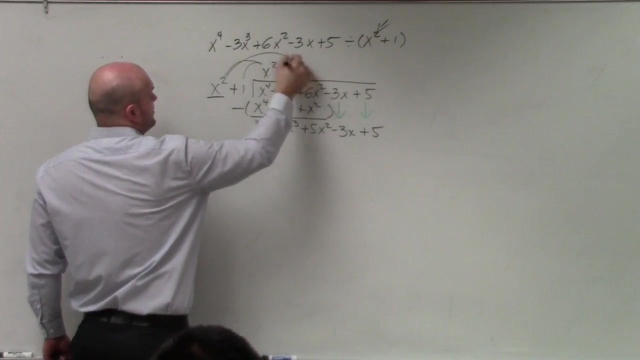 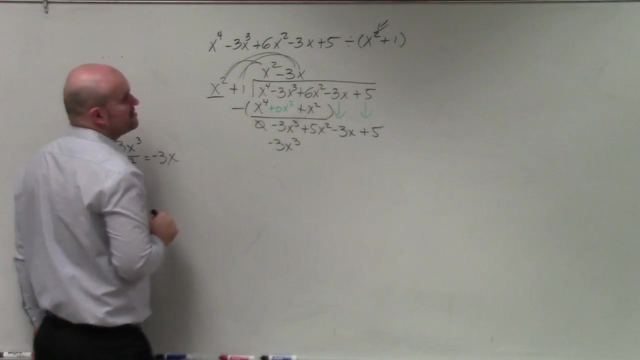 So negative 3x cubed divided by x squared. Well, it goes into there: negative 3x times. Multiply it by both terms again. Negative 3x times x squared is negative 3x cubed. Negative 3x times 3 is going to be a negative 3x Again. I'm going to label it under here, because those